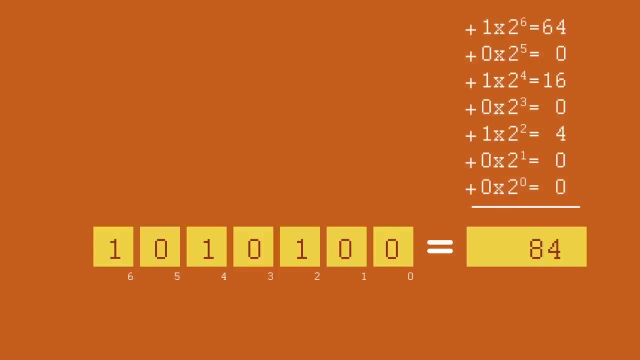 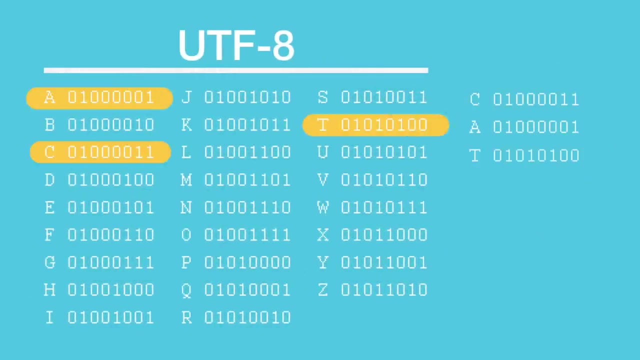 Binary numbered notation works similarly, but with each position based on 2 raised to some power. So 84 would be written as follows: Meanwhile, letters are interpreted based on standard rules like UTF-8,, which assigns each character to a specific group of 8-digit binary strings. 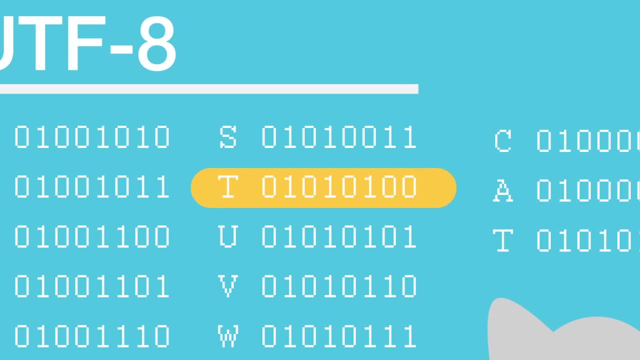 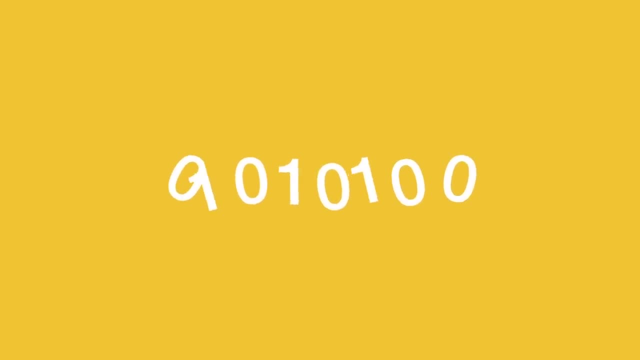 In this case, 01010100, corresponds to the letter T. So how can you know whether a given instance of this sequence is supposed to mean T or 84?? Well, you can't from seeing the string alone, just as you can't tell what the sound da means from hearing it in isolation. 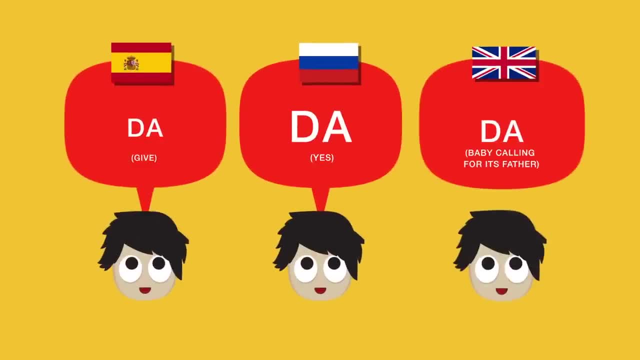 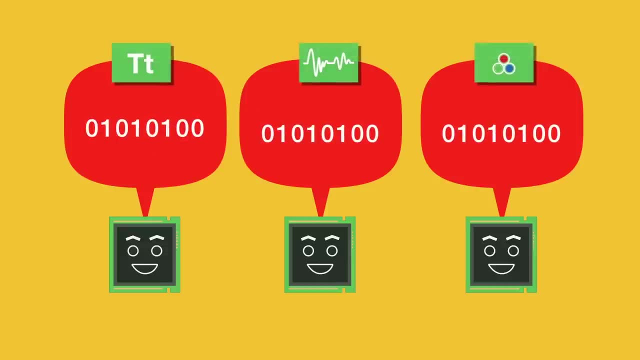 You need context to tell whether you're hearing Russian, Spanish or English, And you need similar context to tell whether you're looking at binary numbers or binary text. Binary code is also used for far more complex types of data. Each frame of this video, for instance. 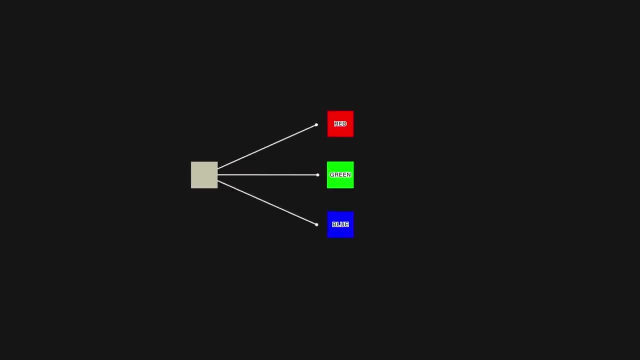 is made of hundreds of thousands of pixels In color images. every pixel is represented by three binary sequences that correspond to the primary colors. Each sequence encodes a number that determines the intensity of that particular color. Then a video driver program transmits this information. 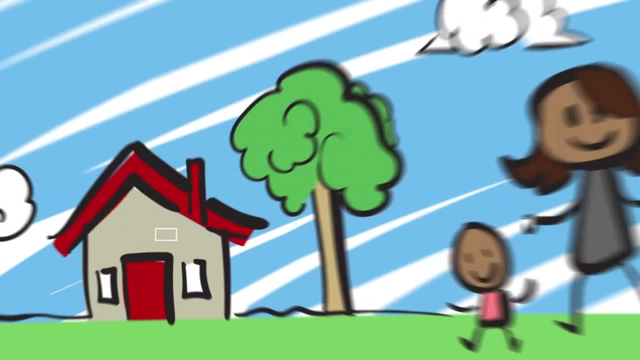 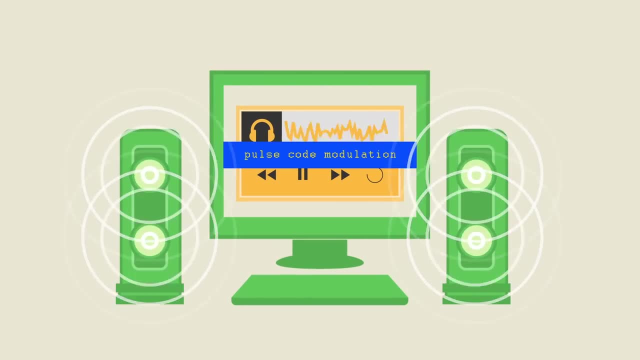 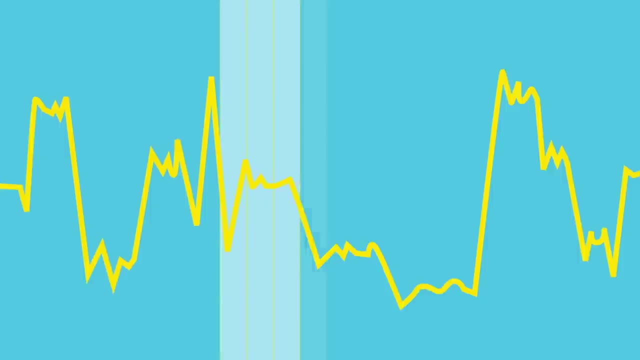 to the millions of liquid crystals in your screen to make all the different hues you see. now The sound in this video is also stored in binary with the help of a technique called pulse code modulation. Continuous sound waves are digitized by taking snapshots of their amplitudes every few milliseconds. 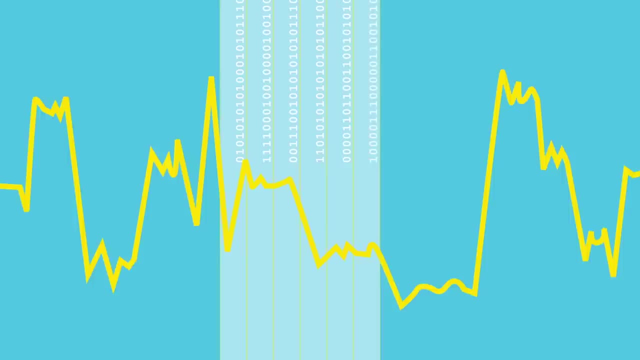 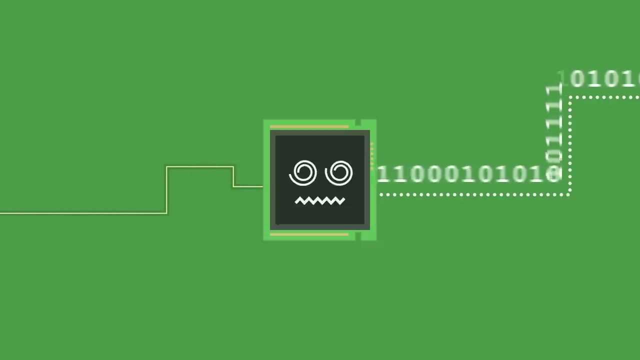 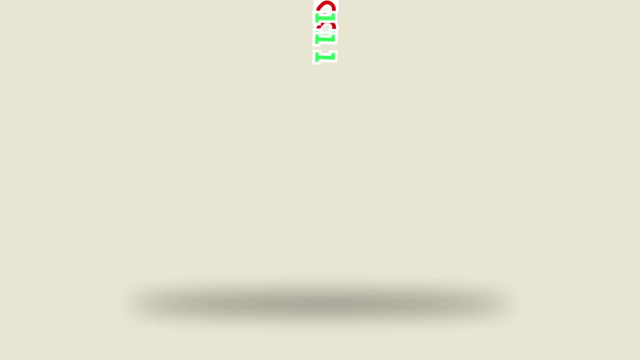 These are recorded as numbers in the form of binary strings, with as many as 44,000 for every second of sound. When they're read by your computer's audio software, the numbers determine how quickly the coils in your speakers should vibrate to create sounds of different frequencies. 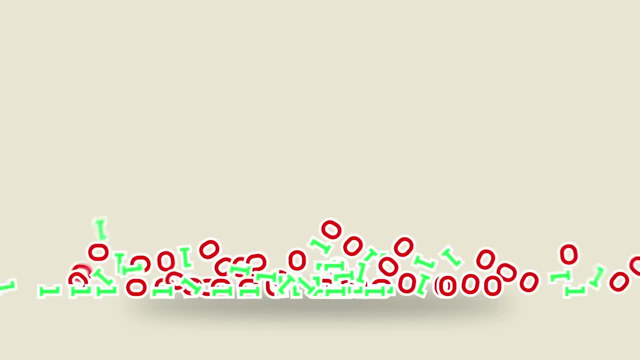 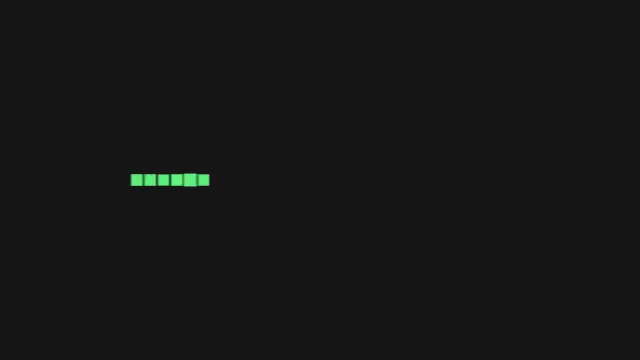 All of this requires billions and billions of bits, but that amount can be reduced through clever compression formats. For example, if a picture has 30 adjacent pixels of green space, they can be recorded as 30 green instead of coding each pixel separately. 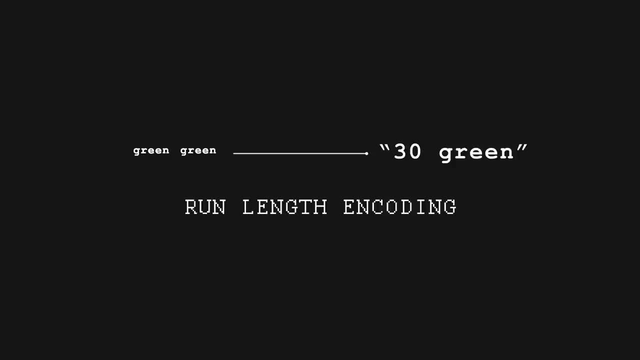 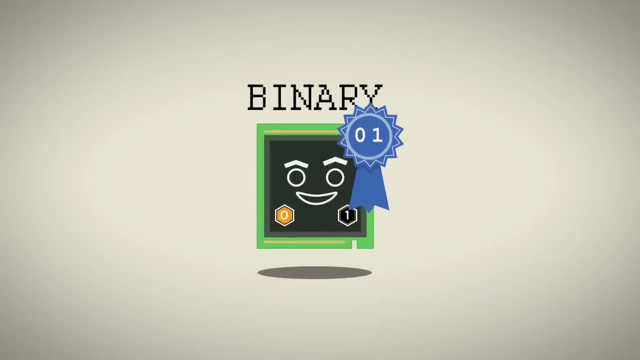 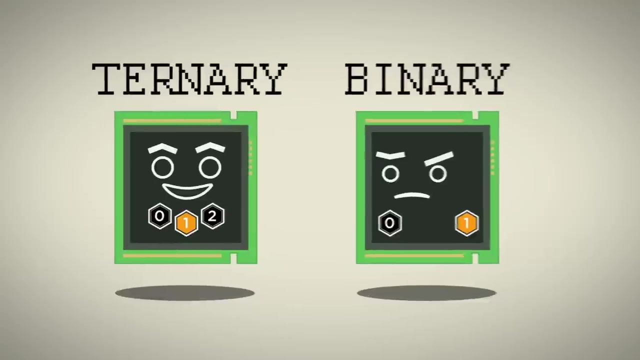 a process known as run-length encoding. These compressed formats are themselves written in binary code. So is binary the end-all end-all of computing? Not necessarily. There's been research into ternary computers with circuits in three possible states, and even quantum computers.